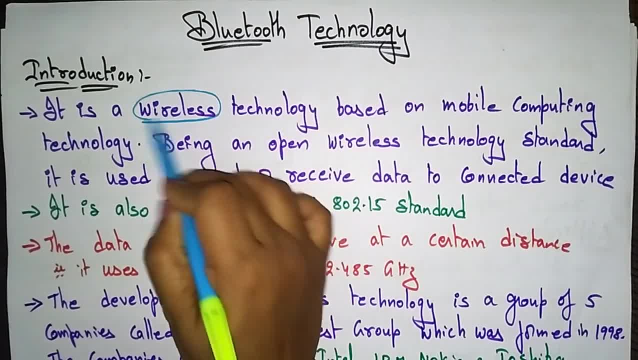 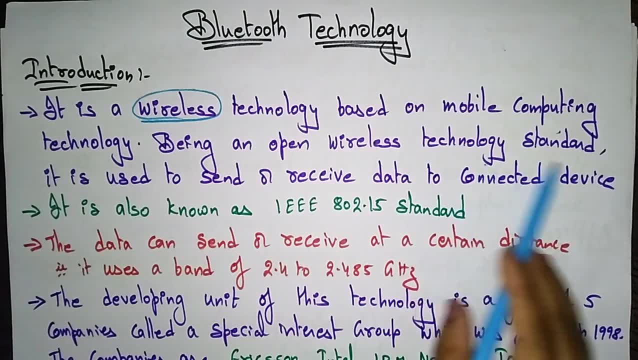 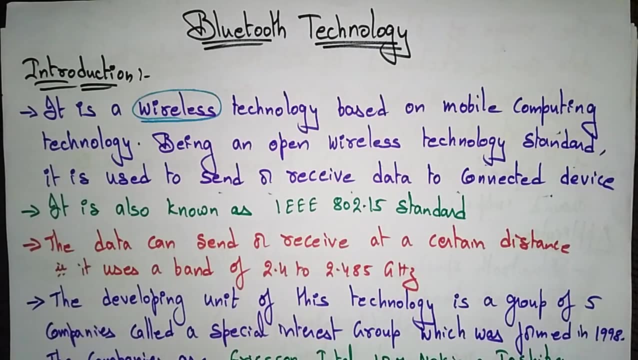 technology. so we know that bluetooth is a wireless technology which is based on a mobile computing technology. being an open wireless technology standard, it is used to send or receive data to connected devices. okay, so because it is an open uh wireless technology standard, what the use of bluetooth technology just to send and receive the data which are connected devices? the thing here is: 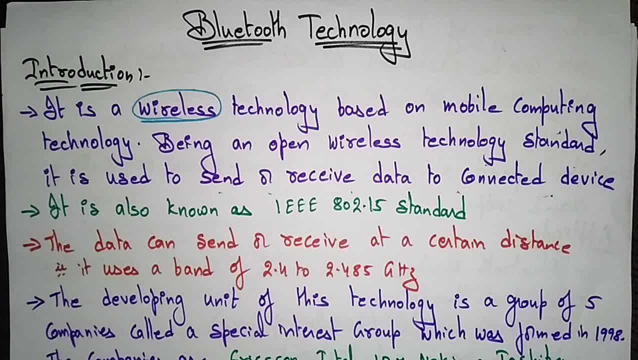 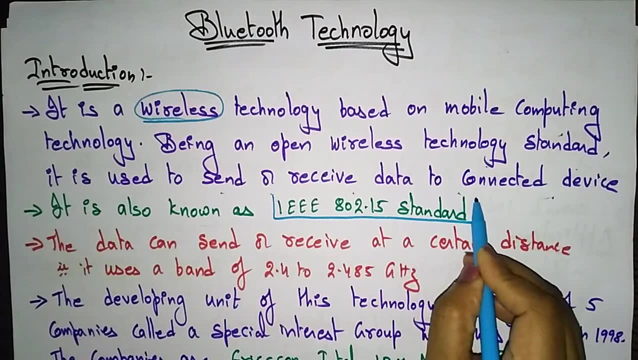 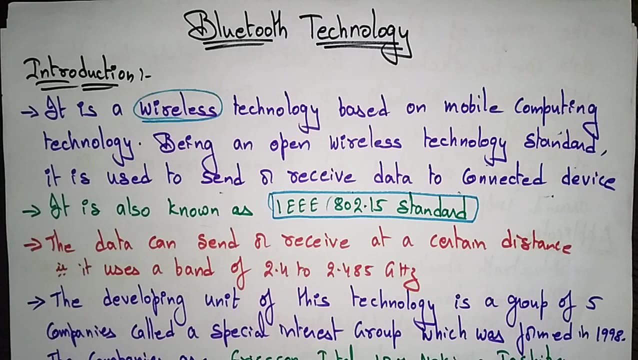 the devices that are connected. for those devices only we can send the data and we can receive the data. so without uh the connections, you can't send and you can't take the data from the unconnected devices. so it is also known as IEEE 802.15 standard. so just remember this uh number. so whenever they are uh, just given uh IEEE 80. write. 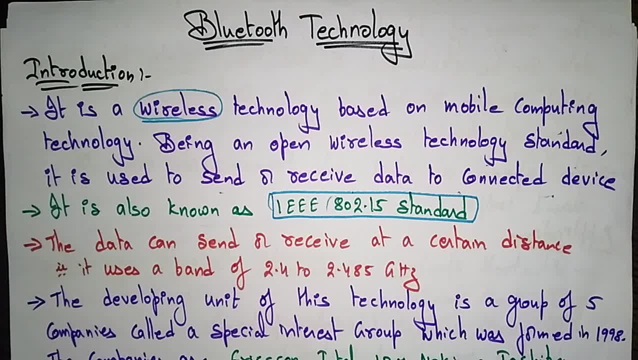 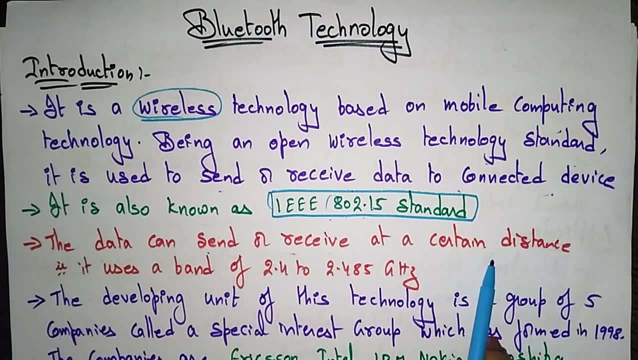 about the IEEE 802.15 standard, so don't confused: 802.15 is nothing but a bluetooth. there's another name for bluetooth is IEEE 802.15. the data can send or receive at a certain distance. that it that is. it is used a band of. 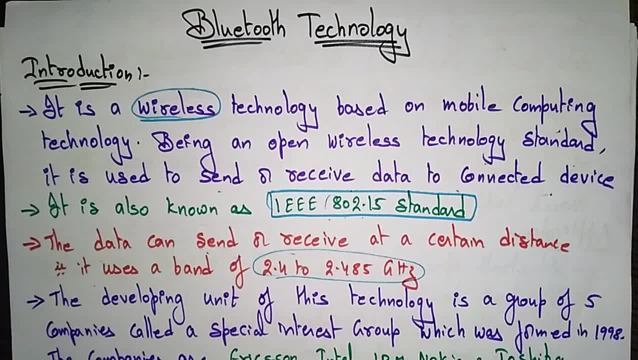 2.4 to 2.485 gigahertz, actually uh, the bluetooth technology. if you take the wireless uh or wi-fi, whatever the technology, it can be ranged. some distance will be there, so based on the bandwidth that is provided by that wireless communication. but here the bluetooth can send or receive the. 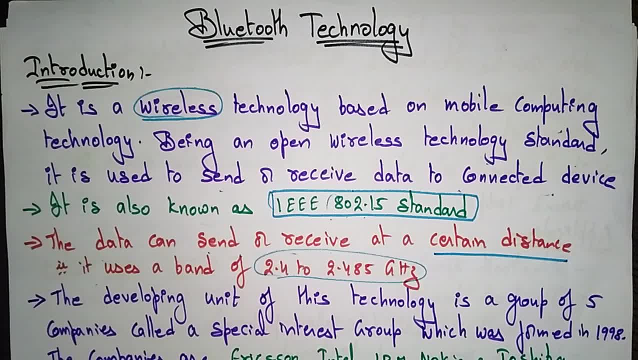 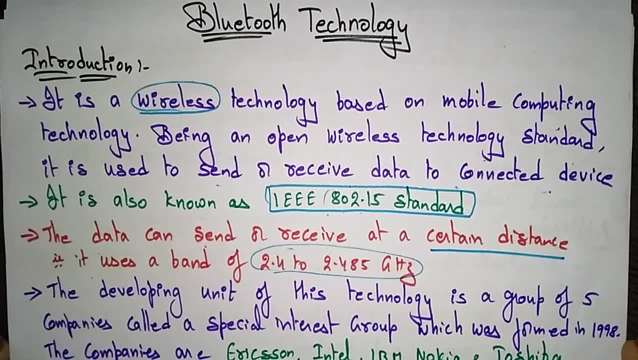 data only to the certain distance, not, it is not supported for the long distance and it uses a band of 2.4 to 2.485 gigahertz. so this is the bluetooth technology. we are saying it is a developing units. why we are saying it is a? 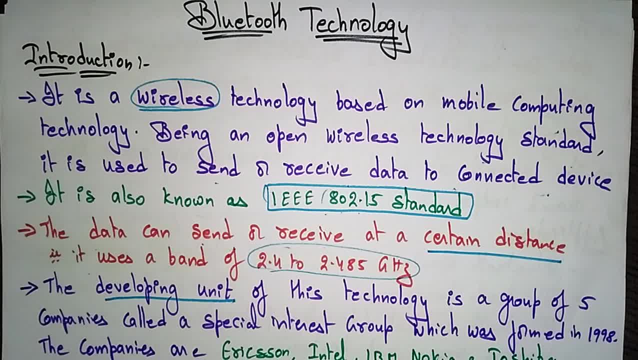 developing unit. it is not the developed one. still some more every year, some more modifications are adding to this bluetooth technology and it is increasing the uh, their distance. okay, so actually, uh, why it is a developing unit means, uh, we are not satisfied to the certain distance we want to be. 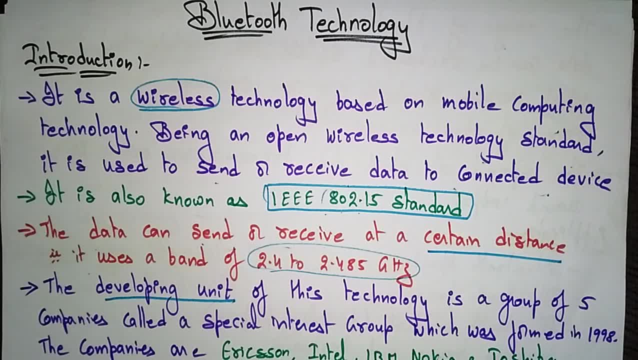 extend the distance of the bluetooth, because the bluetooth technology is a very uh useful technology and it is very simple to implement it, so it's better to make it as more convenient to everyone. so that's why the developing unit of this technology is a group of five. 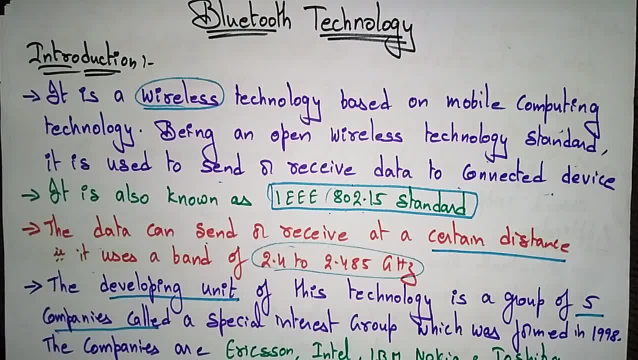 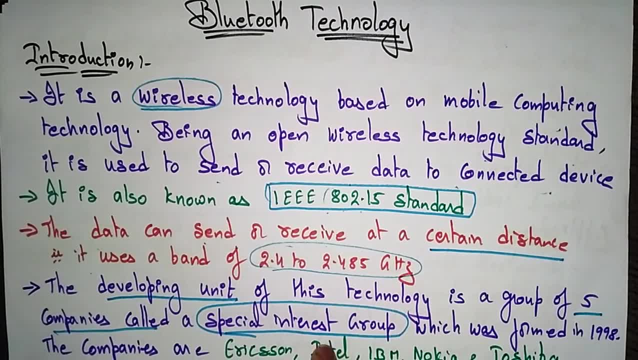 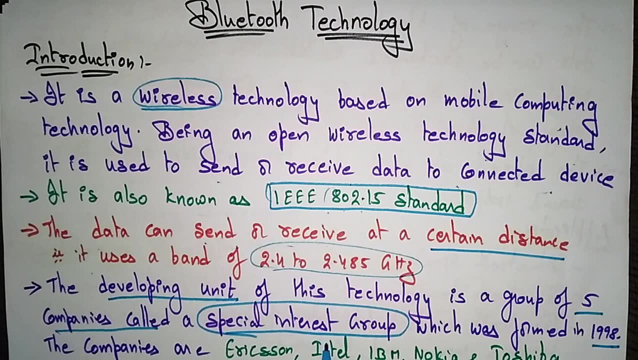 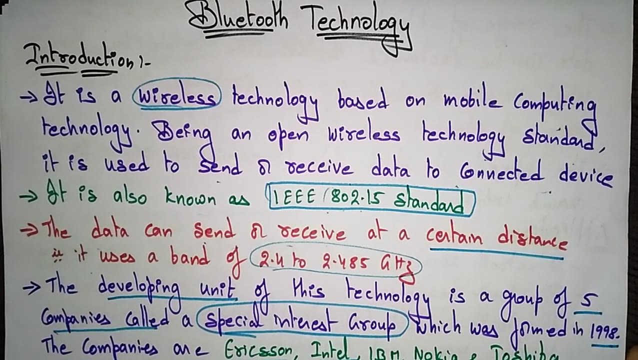 companies, the five companies are developing this bluetooth technology. uh, that come group. you call it as a special interest group, a special interest group which was formed in 1998, the companies that are formed this special interest group, or Ericsson, Intel, IBM, Nokia and Toshiba. so these five companies called as special interest. 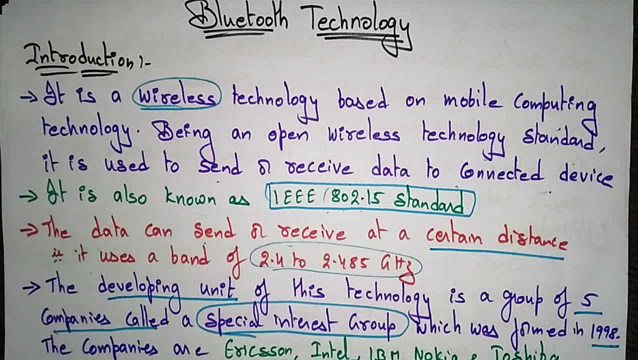 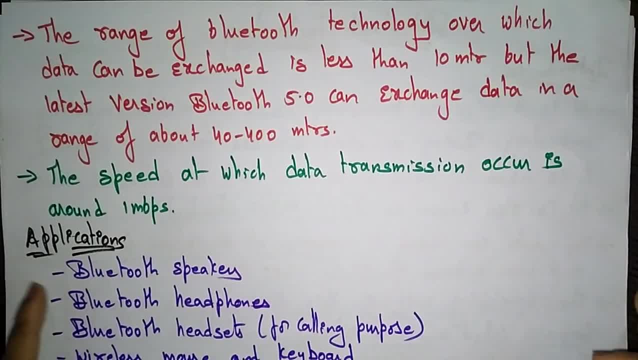 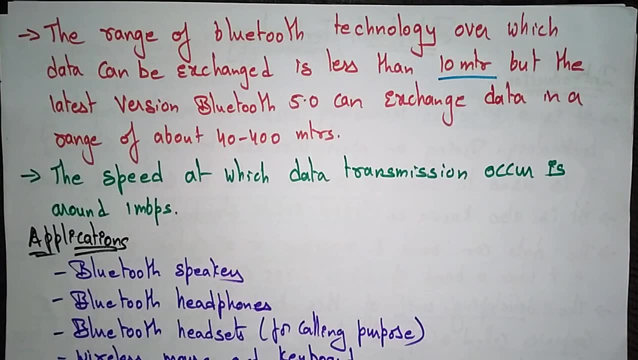 group is formed and these people are working on this bluetooth technology. the range of bluetooth technologies over which data can be exchanged is less than 10 meters. actually, it is the data that can be sent or received is less than 10 meters, but the latest version of bluetooth- 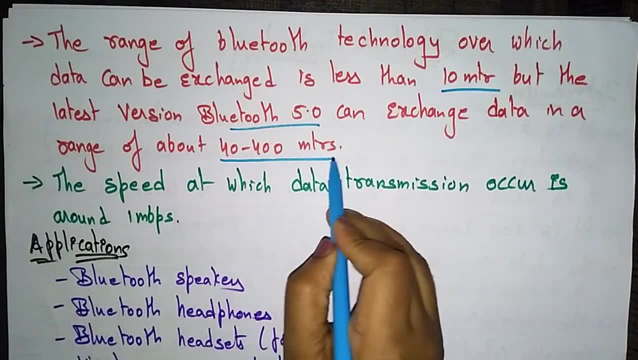 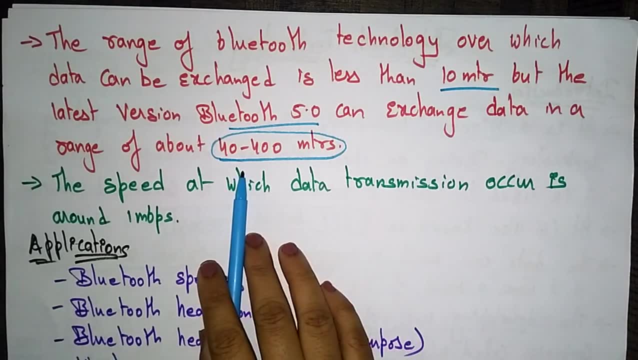 5.0 can exchange data in the range of 40 to 400 meters, so they are still working on that to make this distance to increase. so previously it is only 10 meters, but now the 5.0 version is can exchange the information up to 40 to 400 meters, the speed at which data transmission. 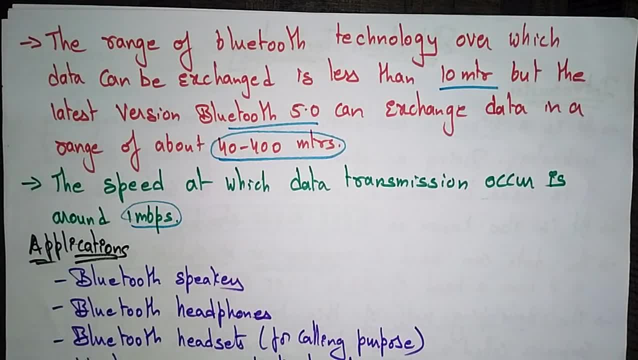 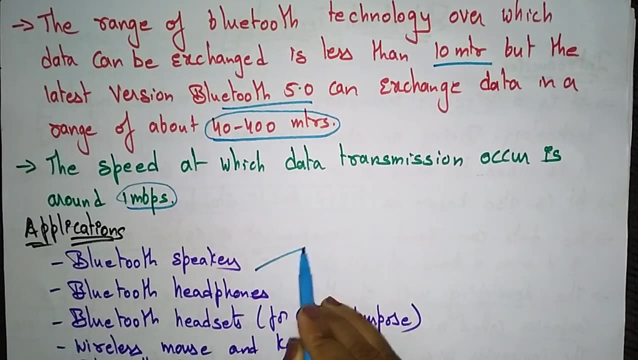 occur is around 1 megabits per second, so the speed is also more. it's just 1 megabits per second. the data is transmitting from source to the destination. okay, so now let's see the applications where this bluetooth technology will be used. the applications are bluetooth speakers are there. 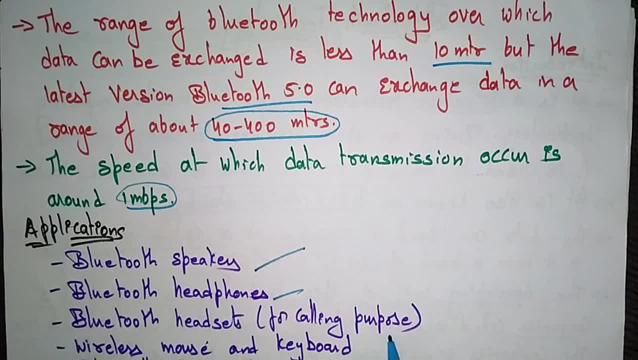 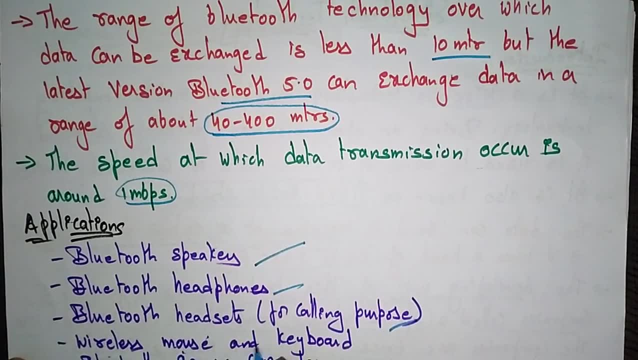 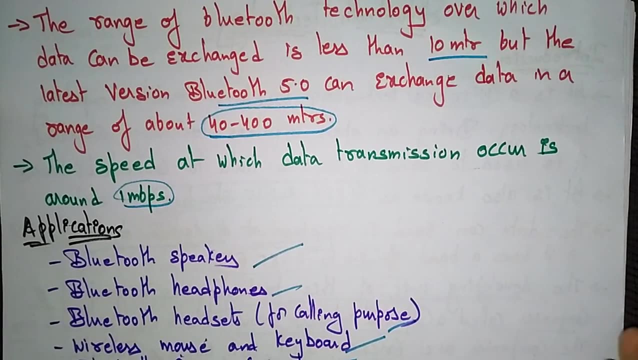 bluetooth headphones, bluetooth headset, which are used for the calling purpose, not the data transferring, so, okay, it's just a calling purpose. headsets, wireless mouse and keyboard. so nowadays everyone is using the wireless mouse and keyboards and the bluetooth gaming consoles, and still so many are there. so these are the applications that are being used for the data transmission.